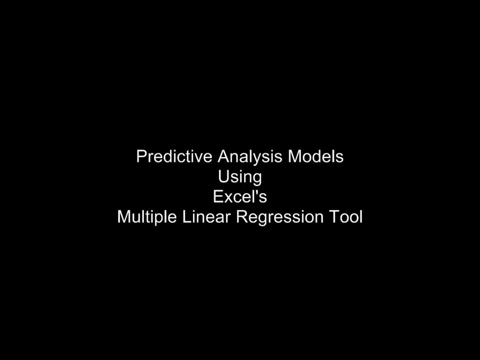 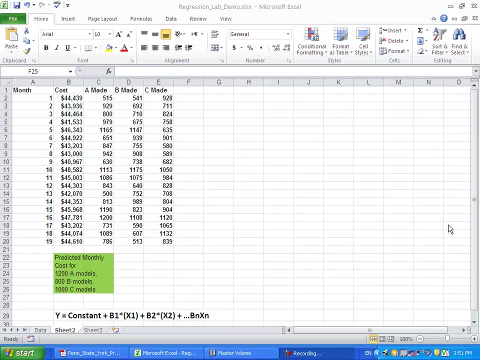 We're going to look at using Excel to do some predictive analysis. We're going to set up a predictive model for our factory and in our factory we make three types of products: A, B and C- And, depending on the quantity of each of those products, is dependent upon how much it costs to run the factory. 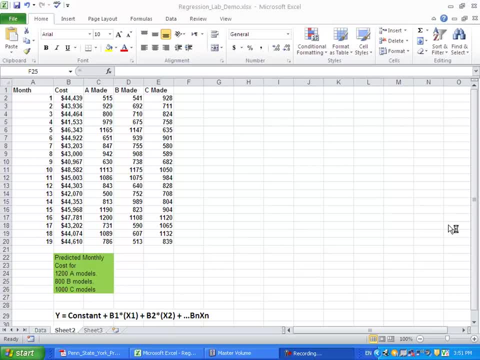 So we've collected this data over the course of 19 months And we're going to use linear regression to do the predictive analysis. Now, in linear regression we have multiple independent variables, And the independent variables that are in this model are the three products we create in our factory: A, B and C. Those are the independent variables. 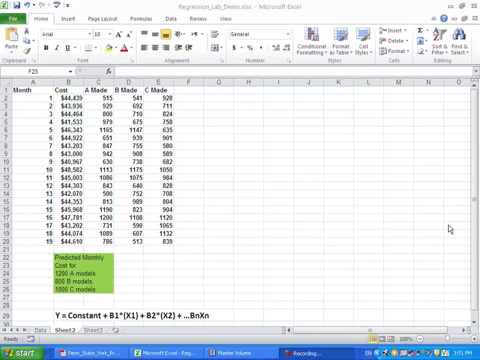 What's the dependent variable? What is dependent upon those three variables is the cost of running the factory. So the dependent variable in this case is the factory cost. So when you look at the regression equation, the multiple regression equation, you will see that what we have is an equation for a straight line And we can assume in this example and all the examples in this course, MIS 204, that there is a loop. 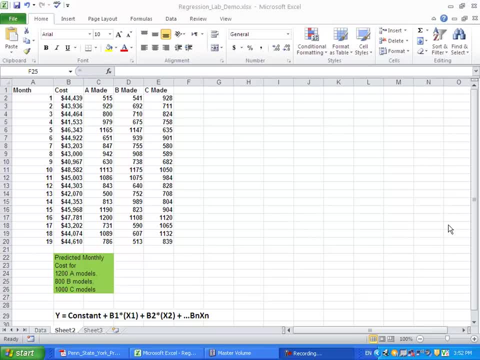 So what that means is that this is a linear relationship, So that's why we're using an equation for a line. So where do we begin in building our predictive analysis model? Well, first of all, we need to make sure that the regression tool is loaded. 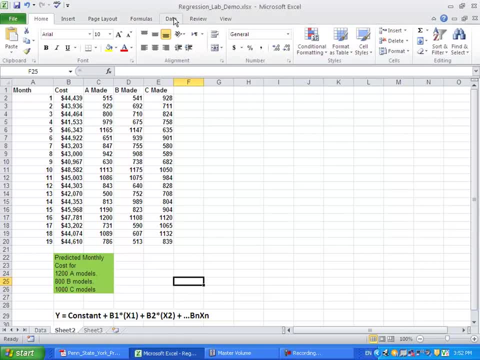 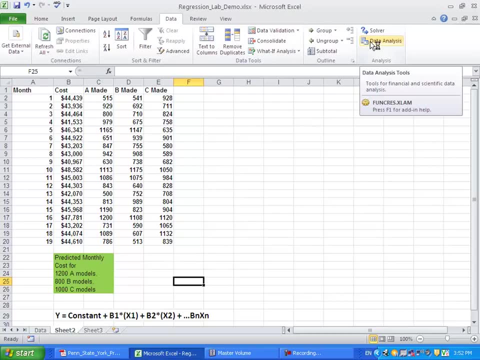 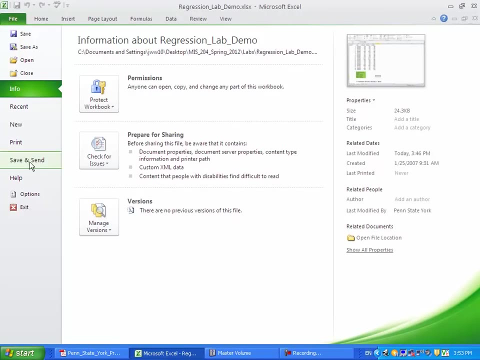 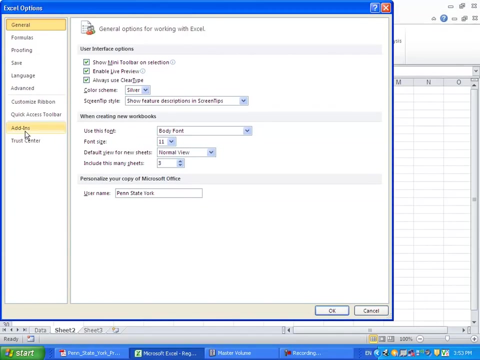 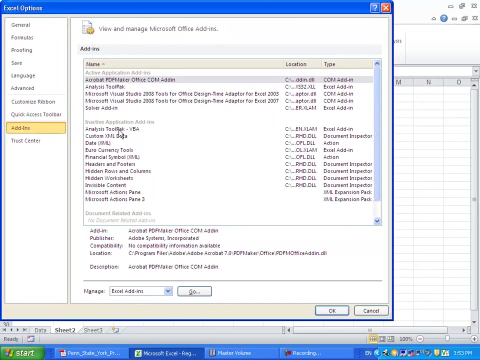 And we go click on data in the tab And when we click on data we see data analysis is loaded. Well, how do we get that loaded? Go over to file. Click options. click add-ins. choose analysis tool pack. click. go. make sure analysis tool. 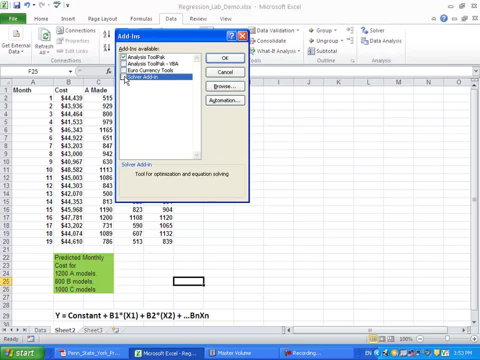 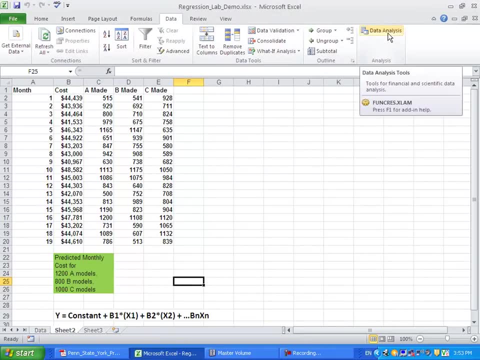 pack is checked. We're not using solver in this particular instance, so we can uncheck that. click okay and the tool pack is loaded. So let's click on data analysis. and when we click on data analysis, we have all of these. 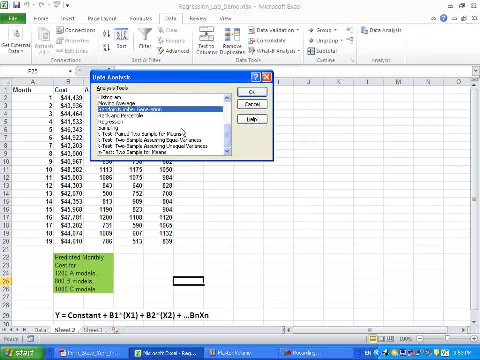 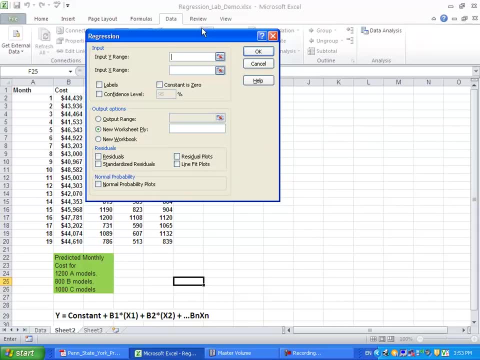 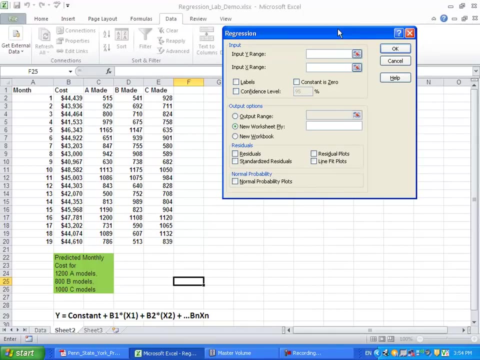 different statistical functions, but the one that we want to use for predictive analysis is regression, So click on regression. okay, Now this dialog box comes up And it's very simple to do multiple linear regression in Excel. The first thing we want to do is we want to select the Y range. 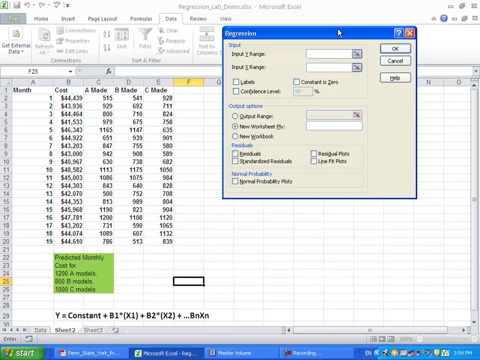 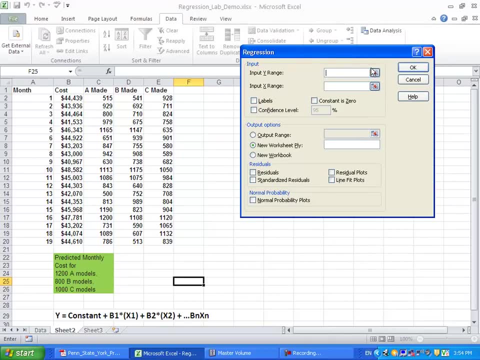 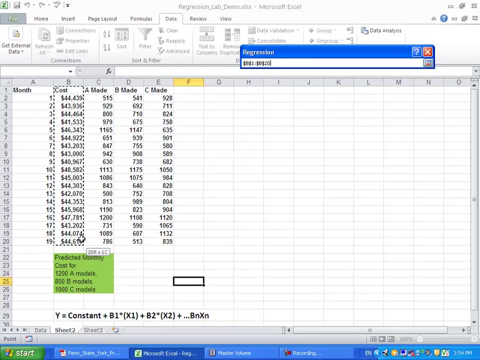 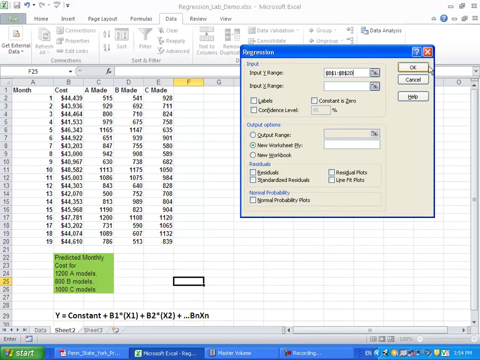 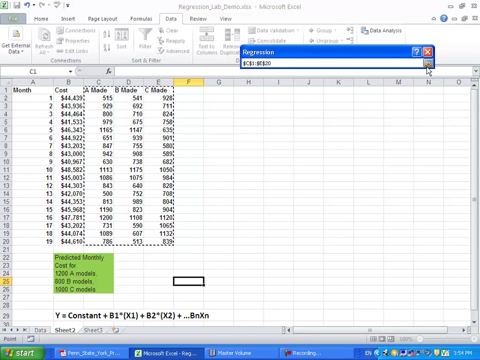 And the Y range is our dependent variable, So we'll select our dependent variable. Cost is dependent upon, Okay, The products that are made in our factory. The X range: we have multiple independent variables. In this case we have X1,, 2, and 3, denoted by products A, B and C. Perfect, 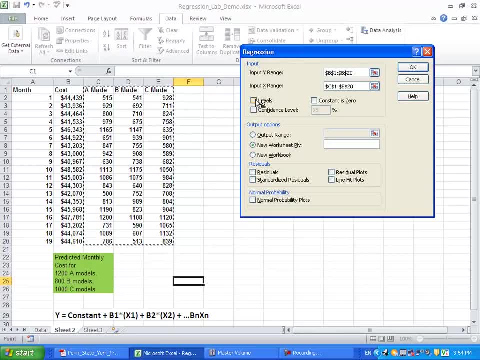 And, if you noticed, I've included the column labels And we're going to have the items. We're going to have the items, All those items together. now we have the statement and we don't have the To do this. here we have Y, and now for the statement. 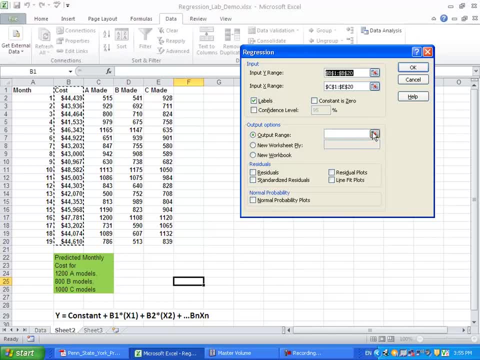 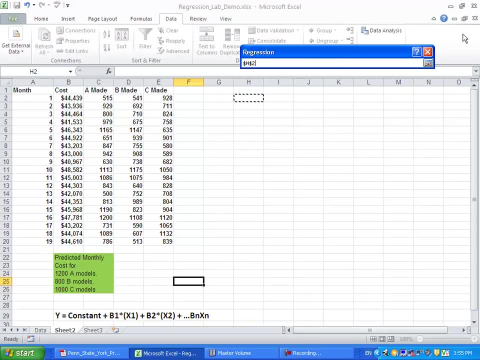 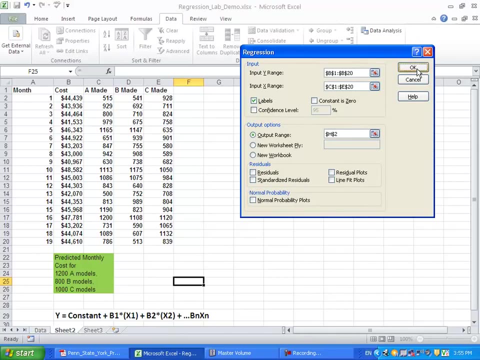 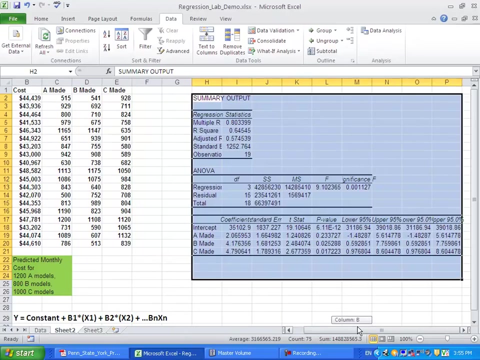 So you can just stick the spelled of Y and U here And For example, the community item is Y. For example, the community item is Y And we'veえば the property item is jakie But the Y, J? 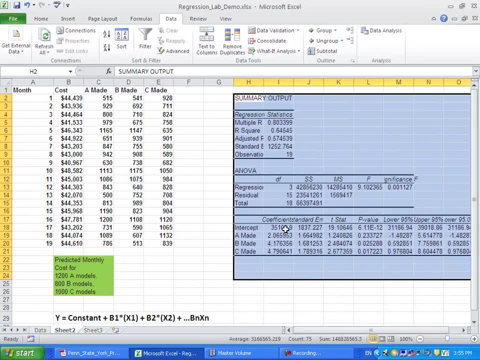 We got, We got Y, And if we brighter on the product, we got Runner J. We have dots on Japan and At the bottom we have the intercept, and the intercept will be the constant in our formula And we have the coefficients for each of our independent variables, which are listed there. 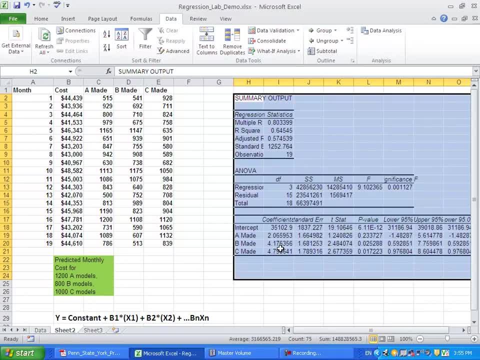 But before we do anything, remember we always need to inspect the p-values, or the predictive values, of each of our independent variables, And any predictive value that is 0.15 or greater we're going to exclude. 0.15 or greater says that the predictive value of that particular independent variable is such that it really doesn't matter in predicting our outcomes. 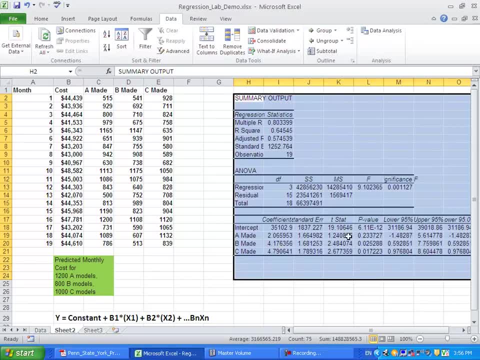 It is not of significance. So when we look at the p-values we see for product A, the p-value is 0.23, which obviously is greater than 0.15.. So we will exclude using the values for the independent variable for product A. 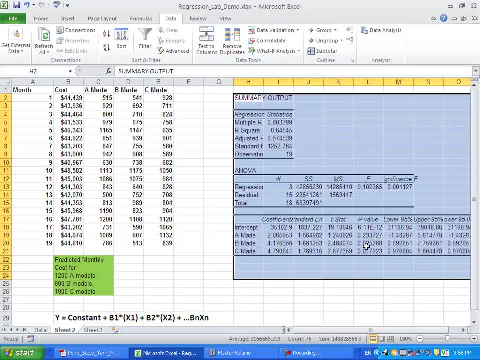 Product B and product C both have p-values well below 0.15.. So their predictive value is much, much greater. So at this point we need to rerun the regression excluding independent variable A. So let's go ahead and do that. 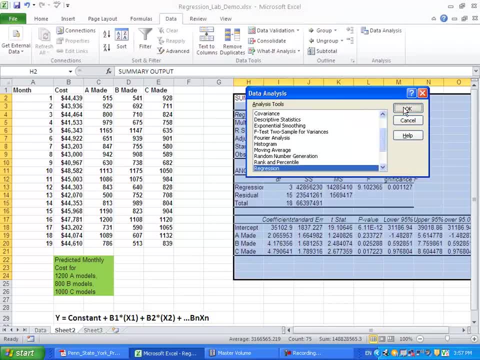 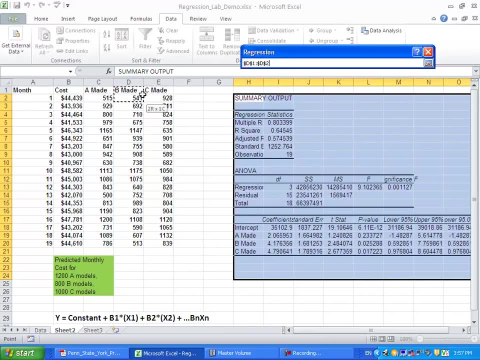 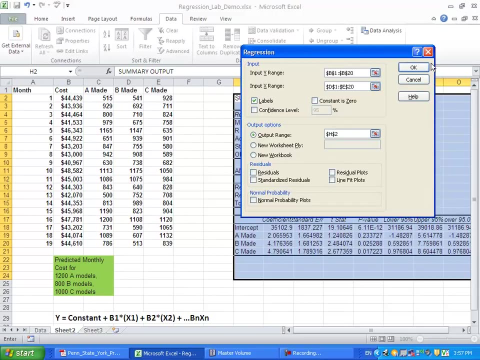 I'm going to go up here, run the regression one more time And instead of selecting A, B and C, this time we're only going to select B and C. Why? Because we evaluated the p-values and found that A's p-value- the predictive value- was just simply too low. 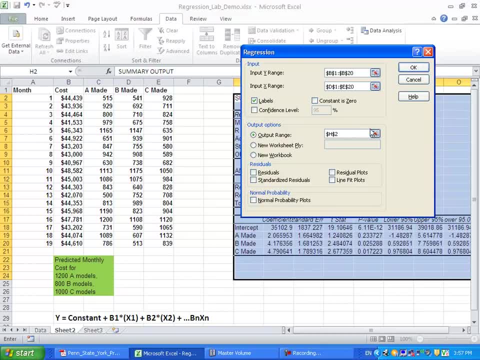 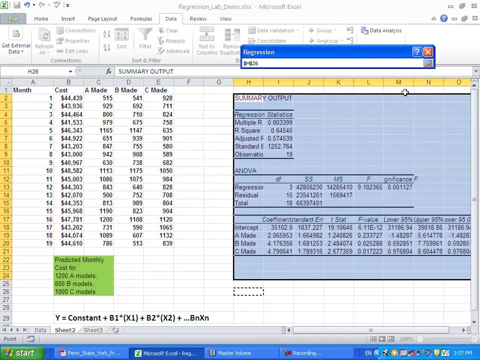 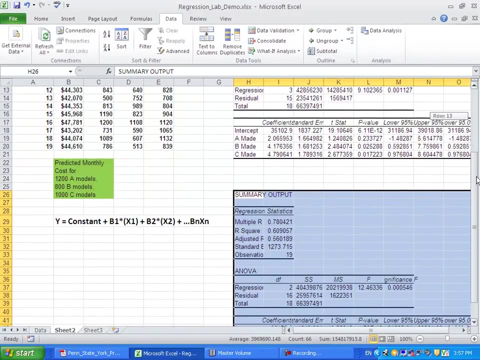 So there we go. We're going to run it again, We're going to put it on the same worksheet. Let's put it down here right below it, And let's click OK And we'll scroll down And Look. 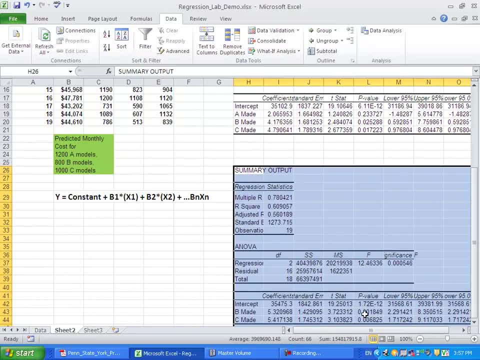 Look at the p-values. Now that we've gotten rid of independent variable A, the p-values, the predictive values of the other independent variables have fallen significantly And they have very, very strong predictive values. So at this point all we need to do is take the different coefficients, plug it into the formula and do our prediction. 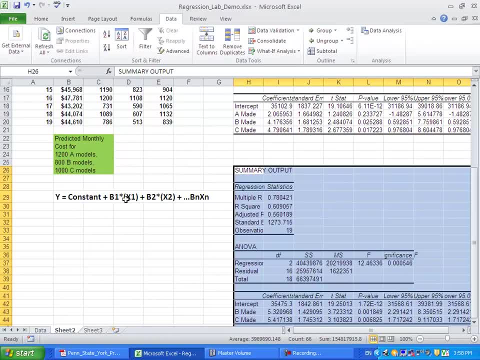 So how do we do that? Well, first of all, let's look at the line formula. The constant is the intercept, The B values is what we're looking for. So in this case we are predicting the monthly cost for our factory if we make 1,200 model A's, 800 model B's and 1,000 model C's. 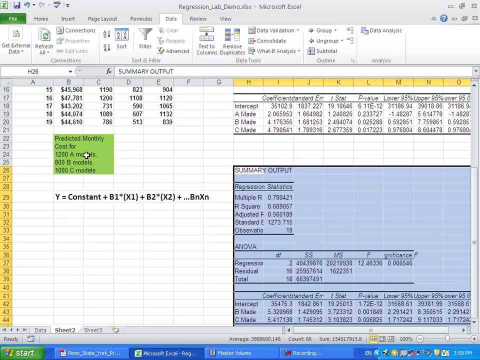 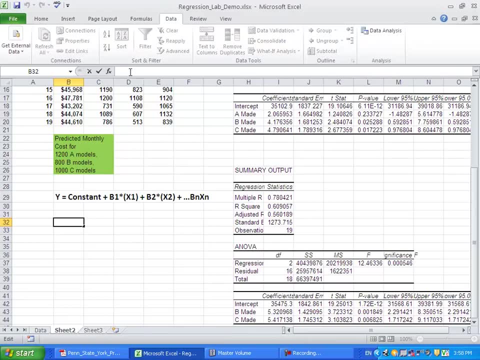 Well, remember we excluded A, so we don't have to include that in our formula. So let's go write our formula, plugging in the variables, And predict our cost. So again, beginning each Excel formula with the equal sign, equals the constant. and I'm reading left to right here the constant which is the line intercept plus I'm excluding A because the p-value was too low: 800 times the coefficient. 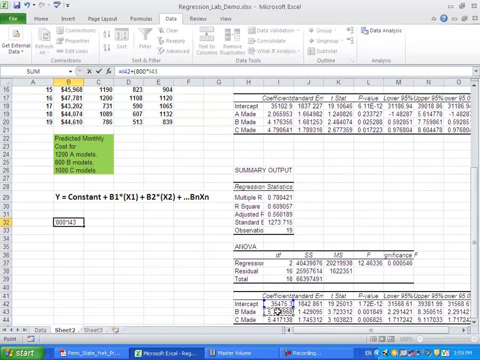 Okay, So we're doing 2000 plus 1,000 times the coefficient for C, And that's it. So let's press enter and make our prediction. And there it is. We can predict that if we made, given our historical data from 19 months, that if we 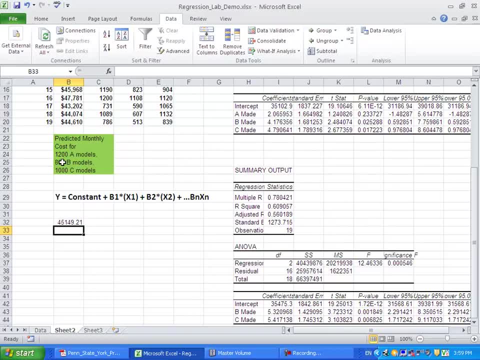 made 1,200 Model A's, 800 Model B's and 1,000 Model C's. it will cost $45,149.21 to run our factory There. it is using multiple linear regression to do predictive analysis.